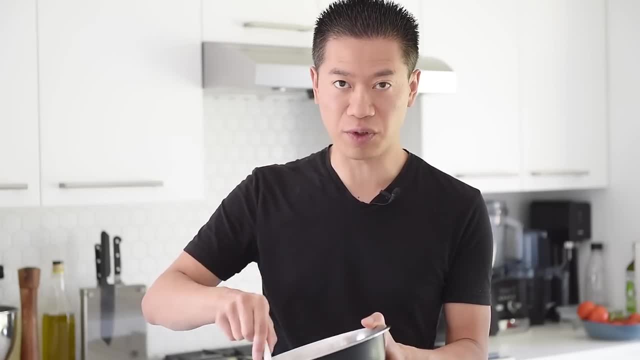 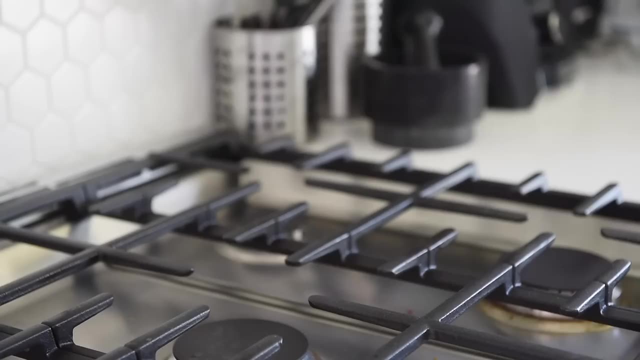 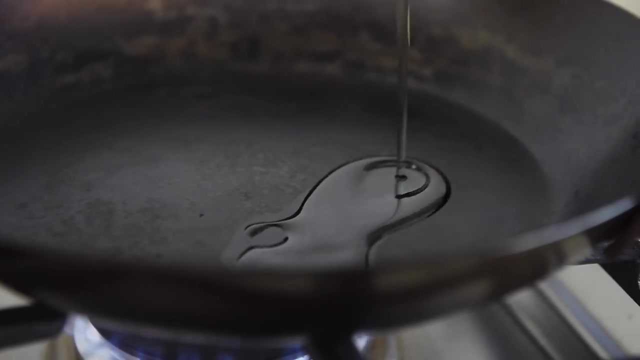 some of that moisture. This way, when you go and stir-fry that rice, you're gonna get a much better result, opposed to having a lot of moisture in that rice. Nonstick pan. Medium-low heat. Two tablespoons avocado oil, Onions and garlic. 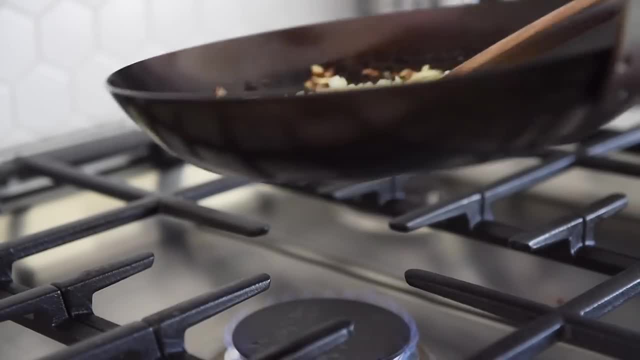 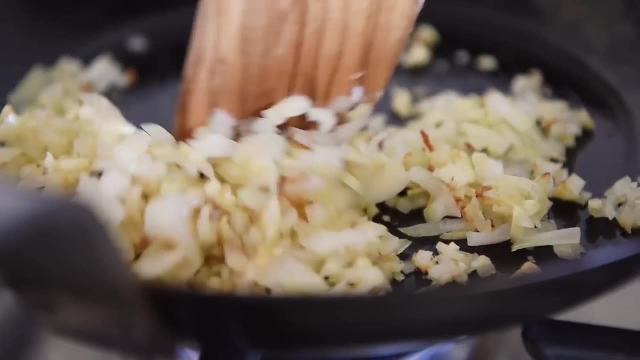 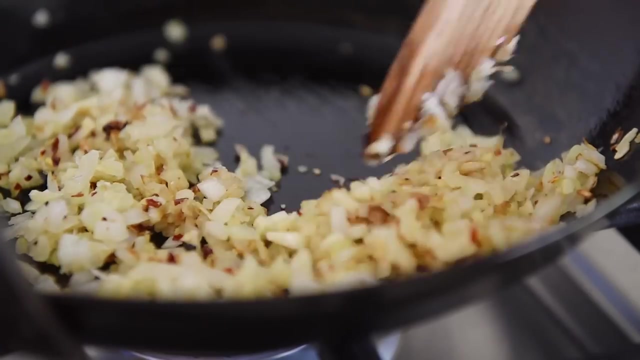 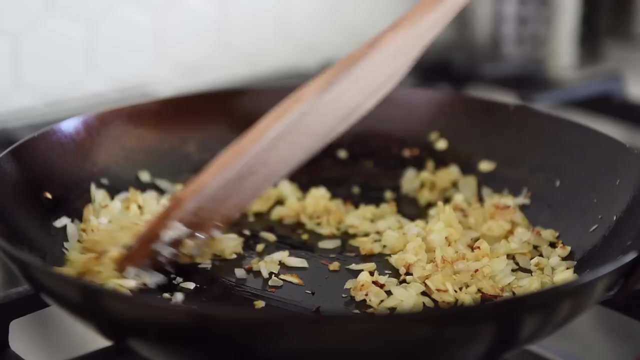 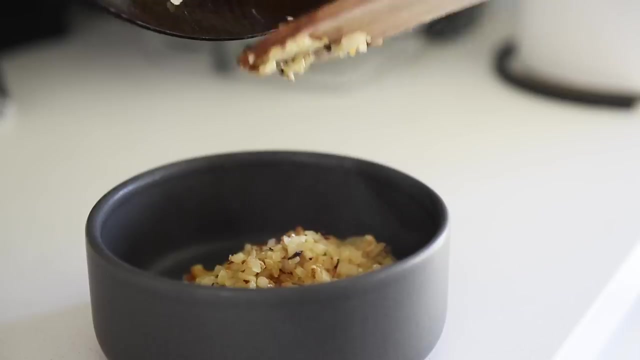 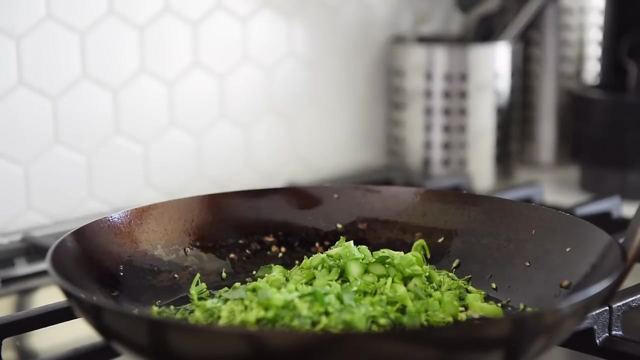 Cook for six to seven minutes. A pinch of crushed pepper flakes. Set aside the garlic and onions. Pan on medium heat with a tablespoon of avocado oil. Broccolini Top with a couple of sprigs of red pepper. A pinch of salt. 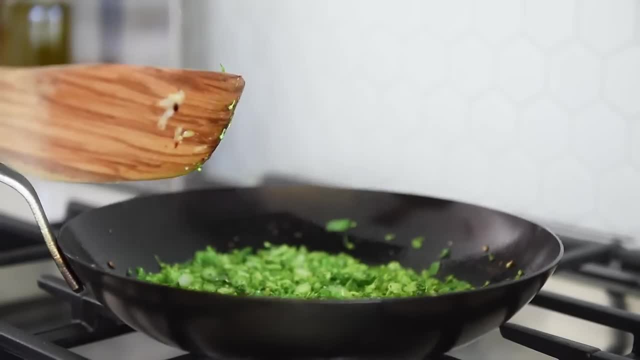 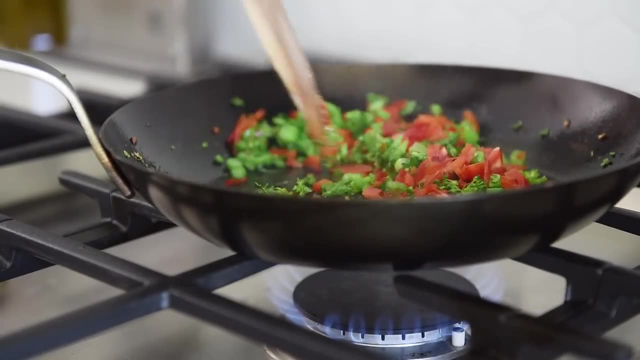 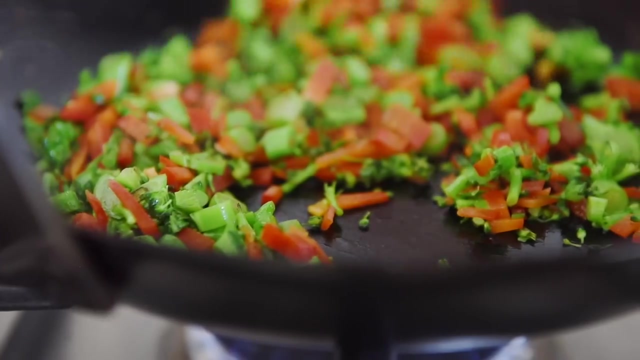 Add a little bit of pepper. Stir fry. Add the onions, Red bell pepper A little bit of later. Sauté for a couple of minutes. sauté for a couple of minutes. Half a cup corn. Half a cup corn. 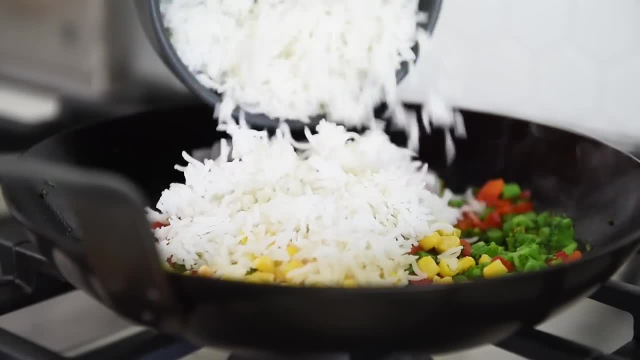 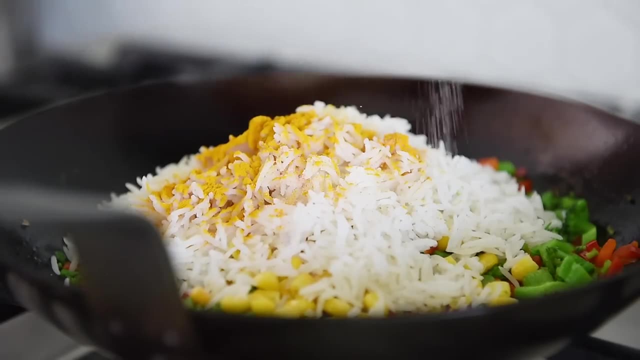 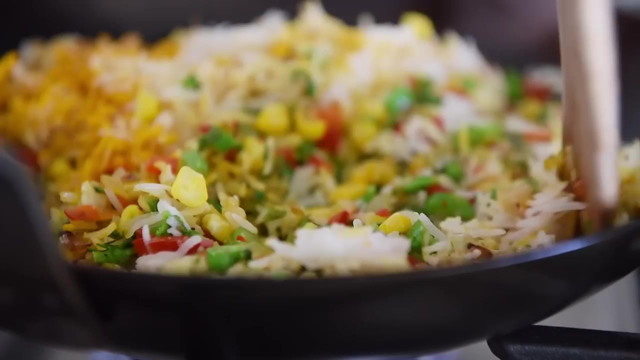 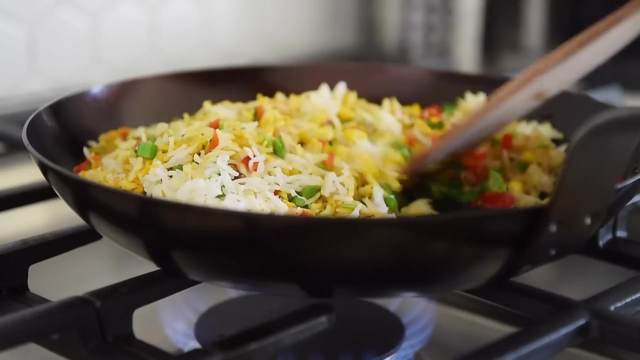 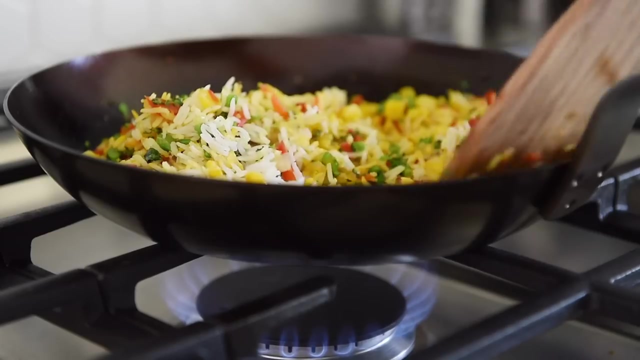 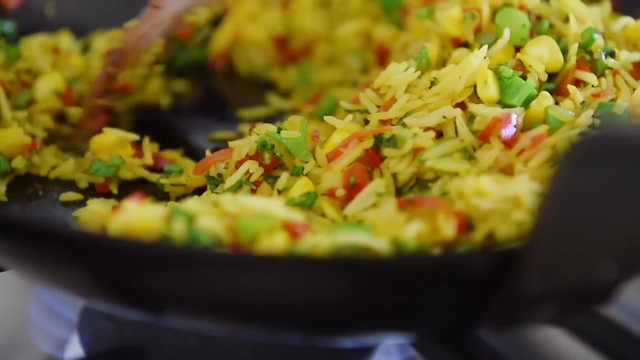 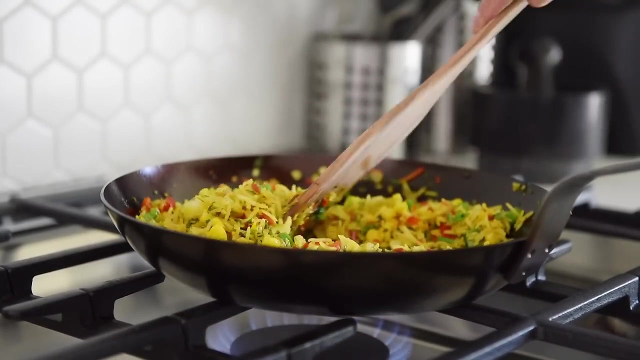 One and a half cup basmati rice. One and a half cups basmati rice, One teaspoon turmeric. One teaspoon garlic. generous pinch of salt. Add back in the onions and garlic. Saute for two to three minutes. Plate. 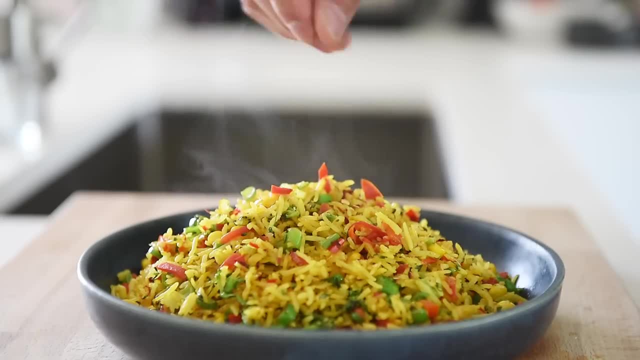 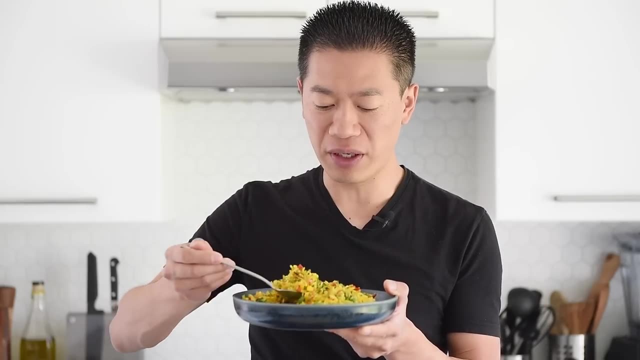 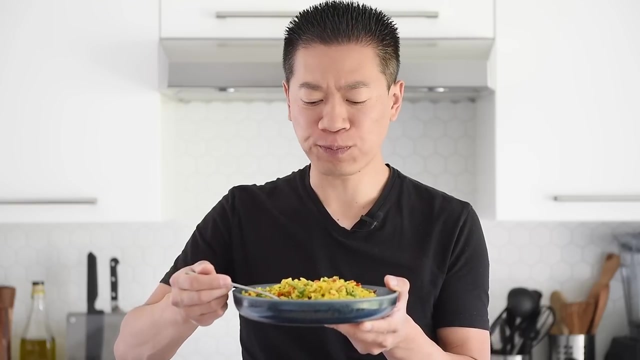 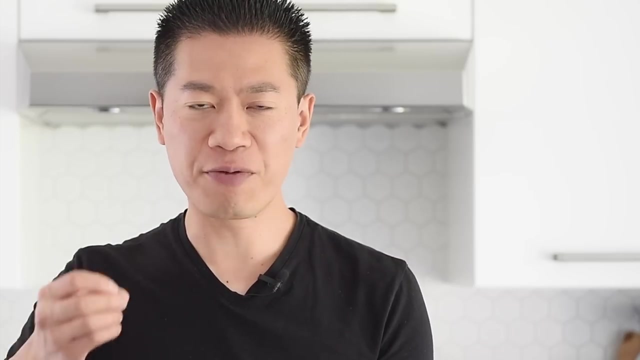 Sprinkle with crushed pepper flakes. You can now make this garlic and rice with absolute confidence. That not only looks amazing, it's going to taste incredible, Because everything was chopped so small. every bite you're gonna get this explosion of flavor. The rice is. 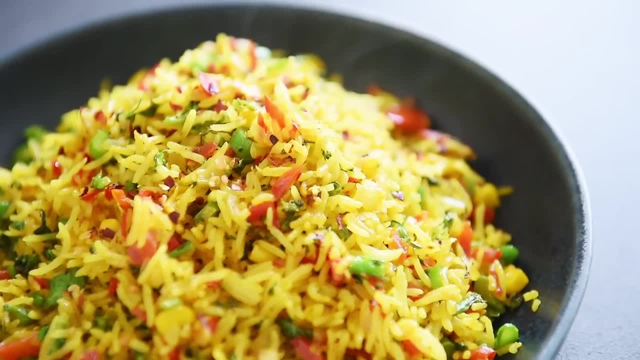 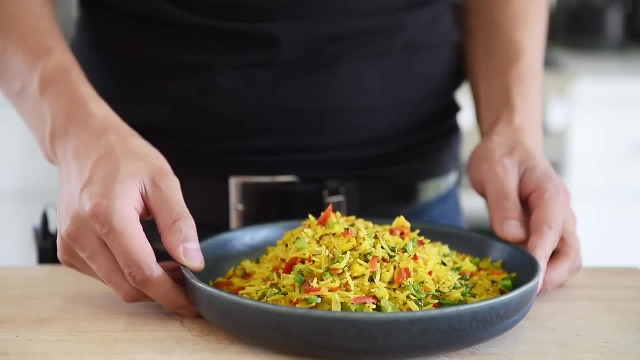 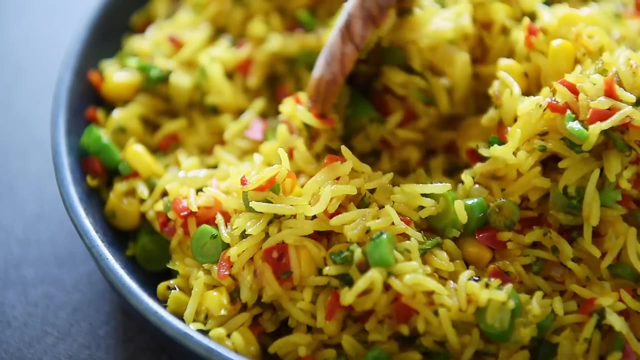 completely coated in this beautiful golden color And when we initially cooked the garlic and the onions on lower heat in that oil, it basically flavors. that oil Flavors the pan with that crazy, incredible garlic flavor. You get a little bit of a kick from that crushed pepper but is balanced out by the 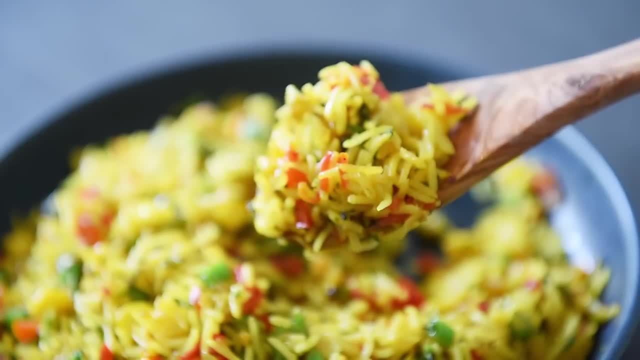 sweetness from that delicious corn. The broccolini just adds kind of a crunchiness and really subsides the flavor of the rice. And that's what we're going to do next. We're going to go ahead and add the garlic and the onions And we're going to 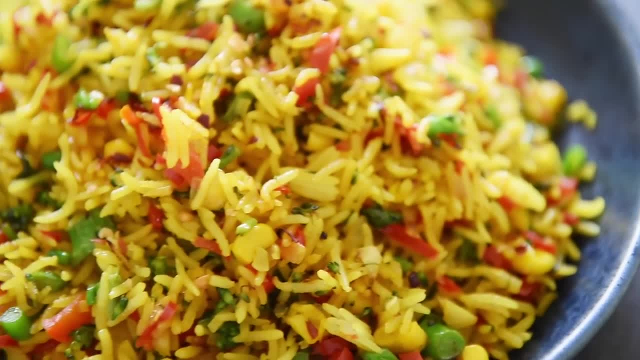 add the garlic and the onions, You can see that the garlic is kind of starting to get a little bit of a brown color and it kind of substantiates this dish. The red bell pepper gives this pop of color, as well as a little bit of 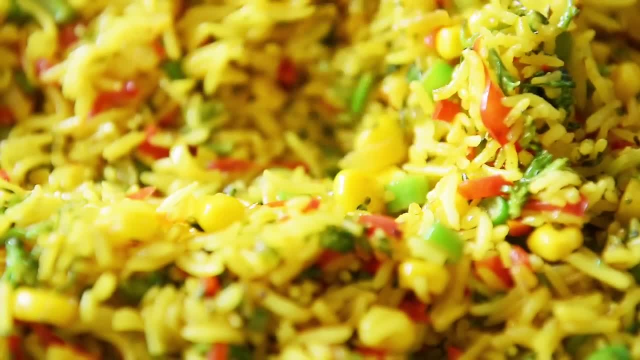 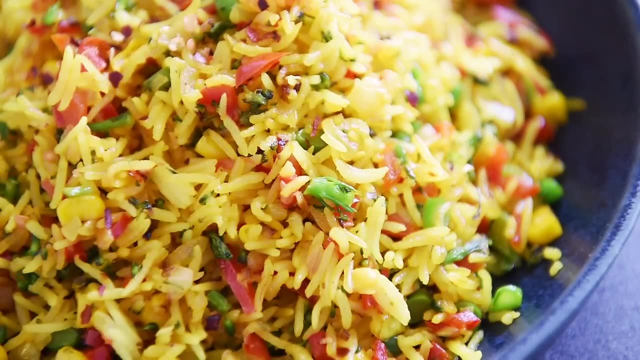 sweetness and a slight acidity as well. It's crazy how there was so much garlic chopped up in this plate of rice, but you can hardly even tell by looking at it, because it just kind of melts into that delicious rice. This is one of those. 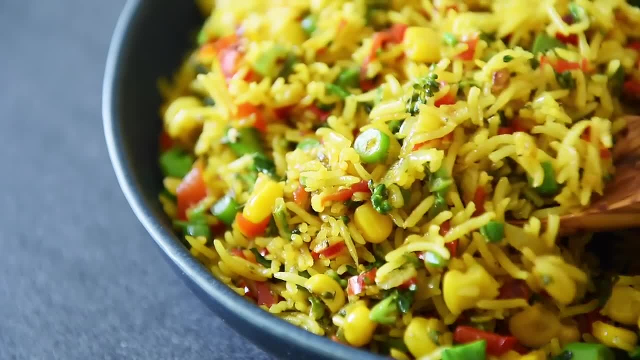 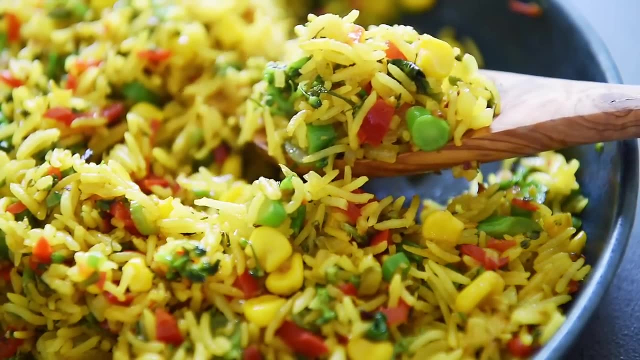 dishes. that's just incredibly savory, Has some deep kind of flavors from the garlic and the onions, Has a little bit of saltiness, Has a little bit of heat, Has that sweetness And you get a bit of that charred flavor from the rice as well. 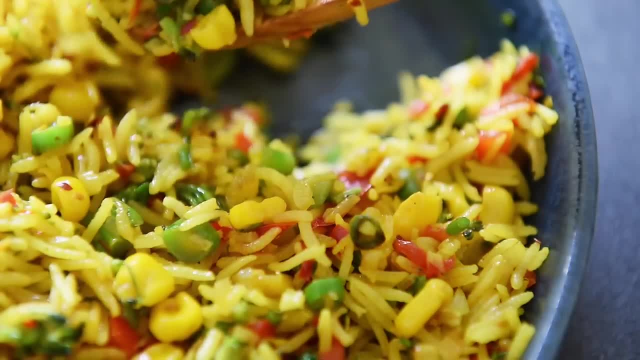 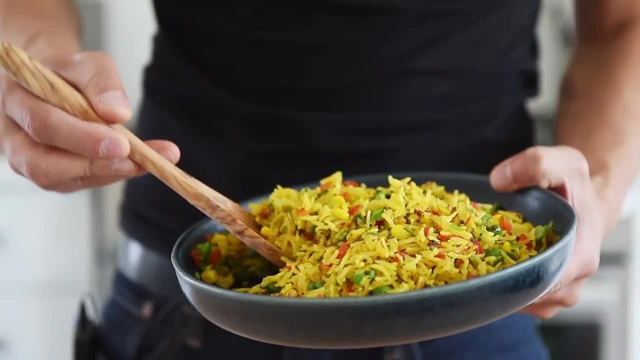 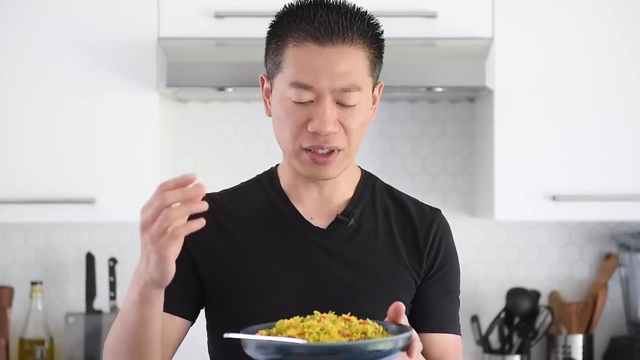 Like I always say, I love turning the kitchen into a restaurant by making these simple but humble, yet beautiful and visually stunning dishes right at home. It's simple, delicious, easy to put together. casual dishes like this. that gets me really excited about cooking. Absolutely love it. 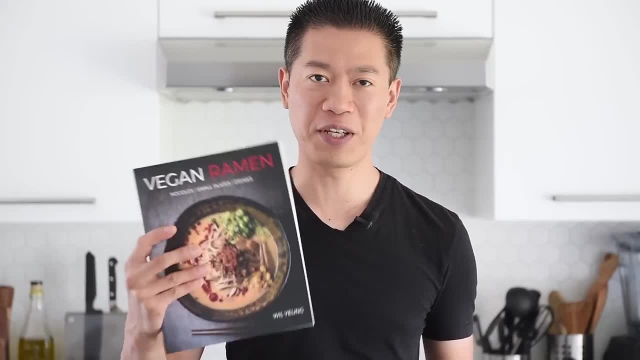 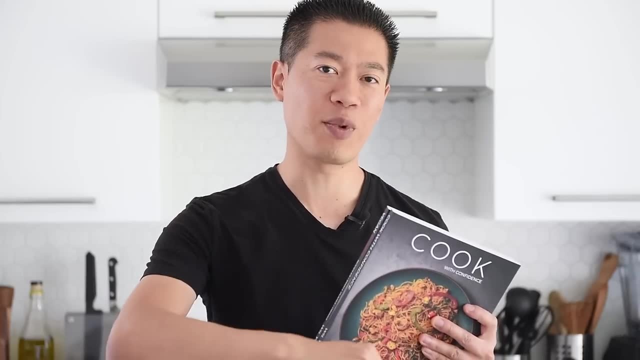 If you love easy and delicious recipes, like I do, then definitely check out the Vegan Ramen Cookbook or the Cook with Confidence Cookbook To take a sneak peek inside the book or to order your signed copy. I'll leave a link in the description box below for you to check that out. As always, remember to subscribe, hit that. 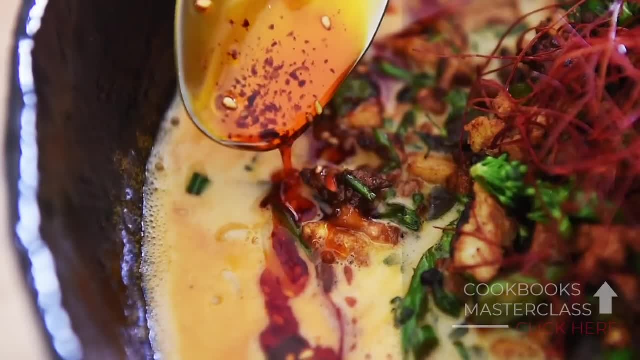 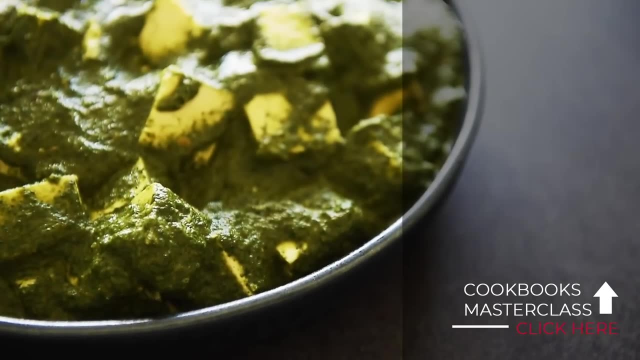 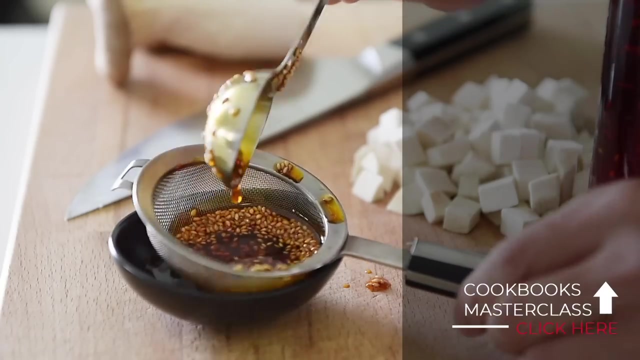 notification bell and I'll see you in the next episode. Thank you so much for watching and I'll see you in the next one.